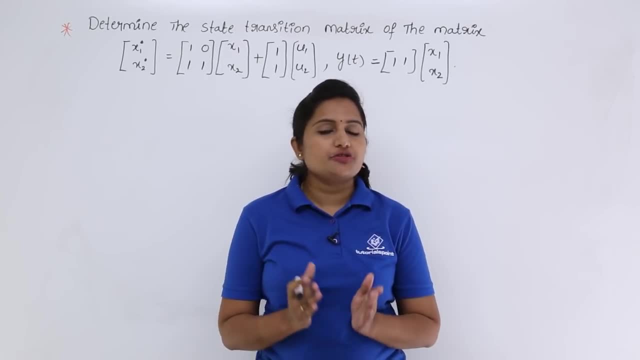 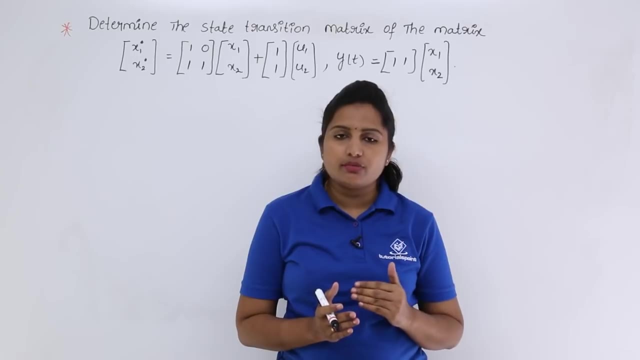 In this video, we are going to solve a problem related to state transition matrix. Up to now, we discussed about how to analyze a system by using state space analysis, and we already derived this equation for state transition matrix in the previous classes. With that knowledge, we are going to solve this problem. 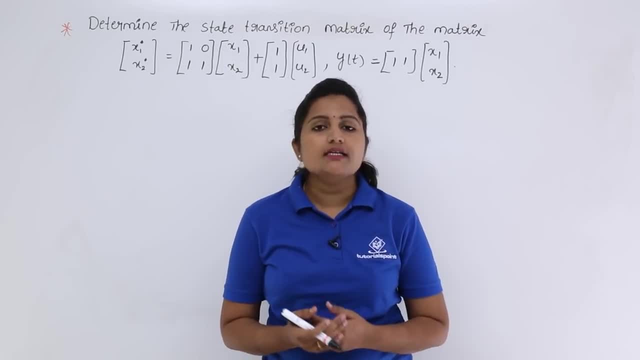 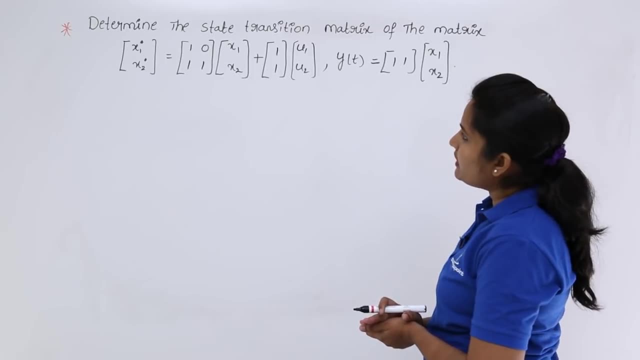 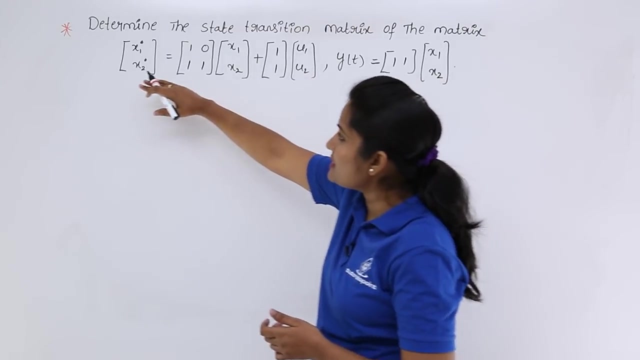 Here we are going to find state transition matrix for the state model given. So here the problem is like this: determine the state transition matrix of the matrix given. So this is the state model. If you observe, this is x, dash and this is x and u. So 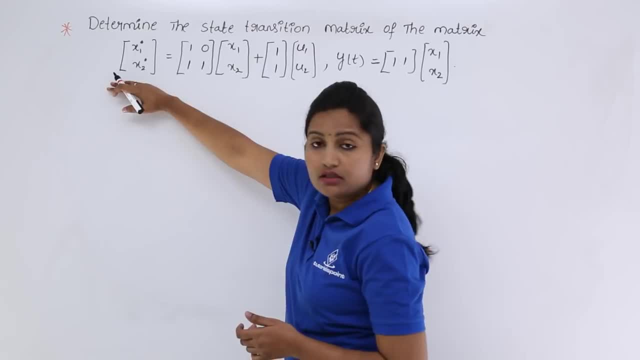 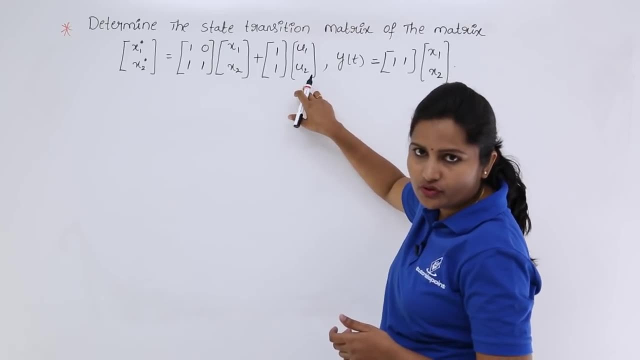 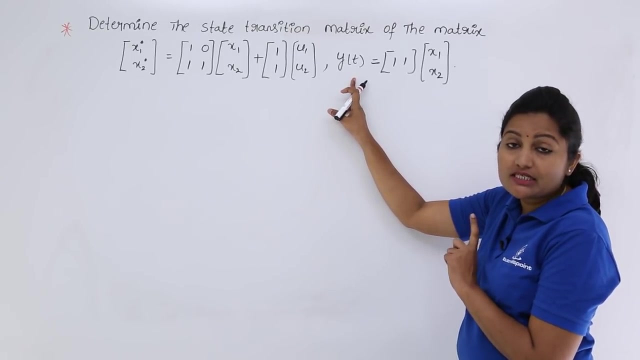 this is the state equation. So here this is nothing but x. dash of t is equivalent to a into plus b into u. So this is nothing but state equation. and where you are having equation with y of t, that is nothing but output equation. These two are said to be state model For this. 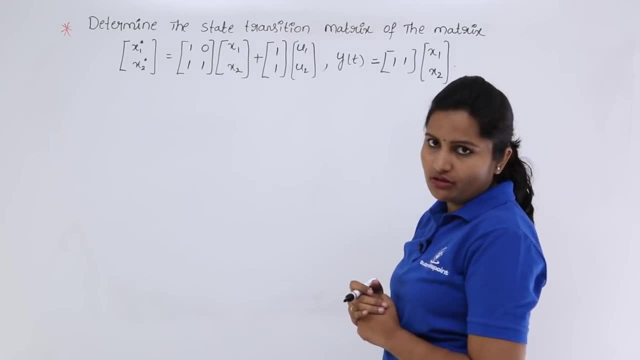 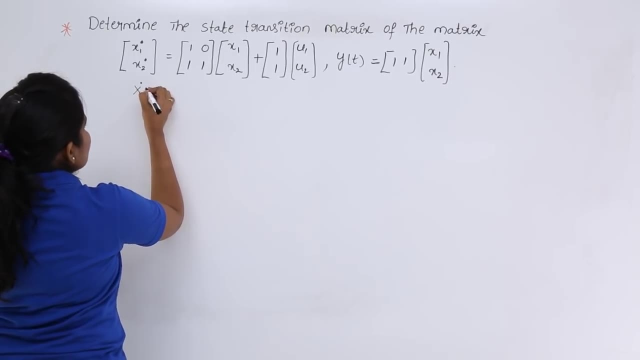 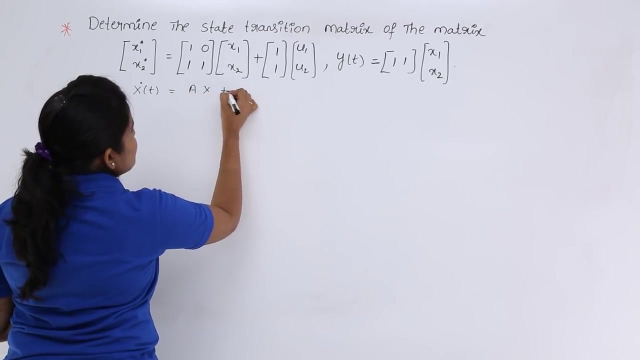 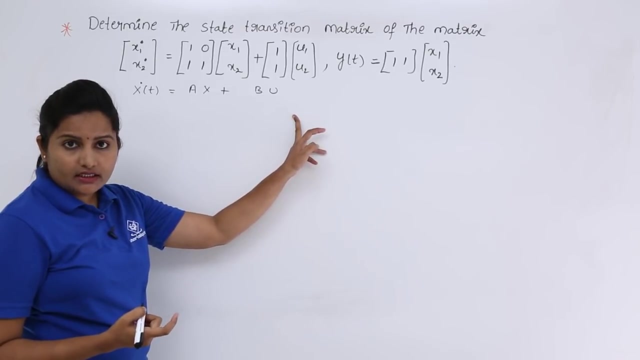 state model. we need to find state transition matrix. So now I am just writing for your reference. This is equivalent to x. dash of t is equivalent to this is a into x plus b into u. So if you see, this is state equation. If you see this is y of t is: 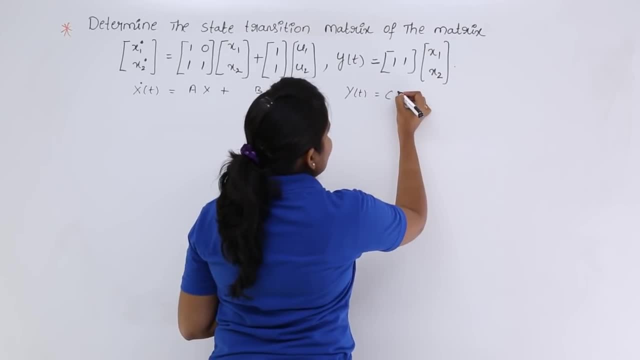 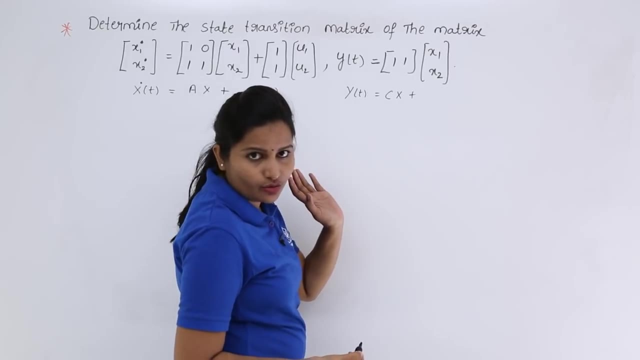 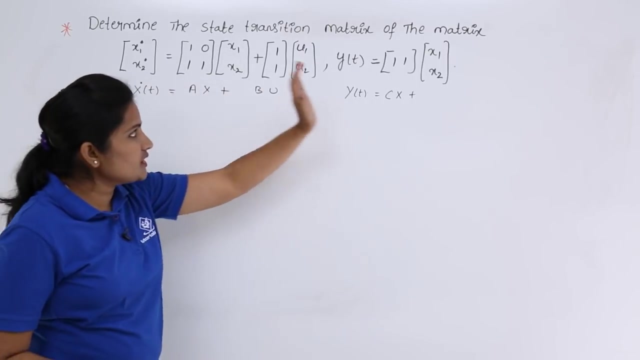 equivalent to So c into x plus d into u should be there, but in the given equation that is 0, d into u of t is equivalent to 0. So here this is state equation and this is output equation. that is ok, but we need to find state transition. 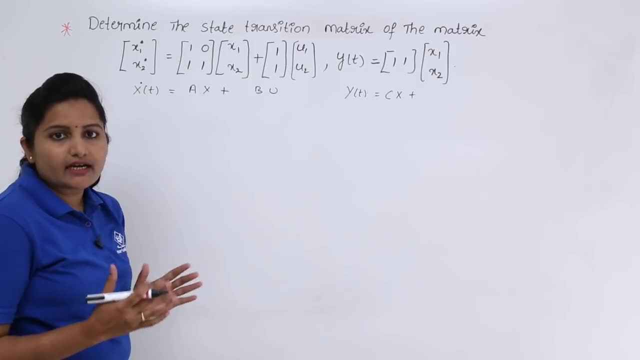 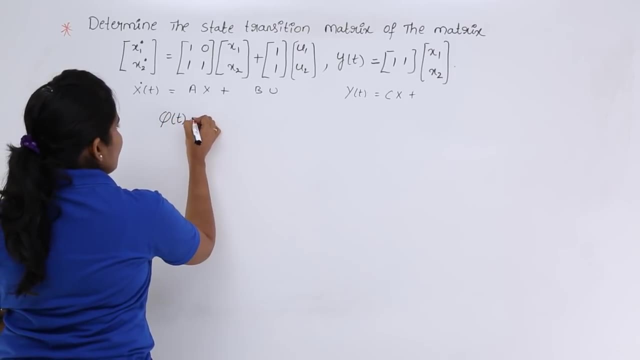 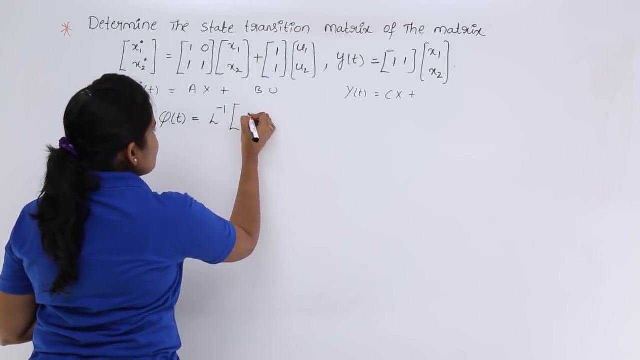 matrix. From the previous video we can write the equation for state transition matrix like this State transition matrix we represented with phi of t. For this phi of t we derived state transition matrix equation as inverse Laplace transform of S, i minus a whole inverse. So this is: 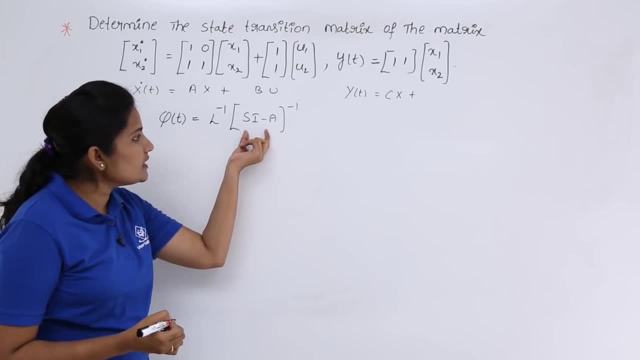 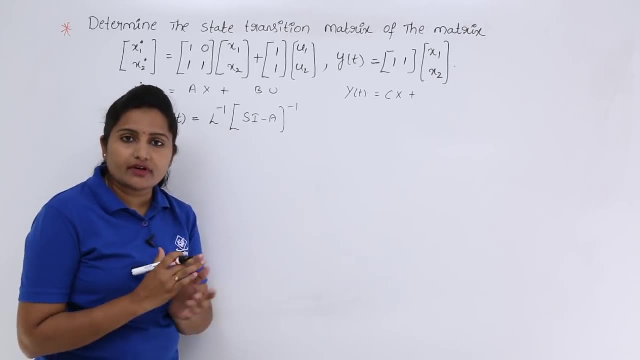 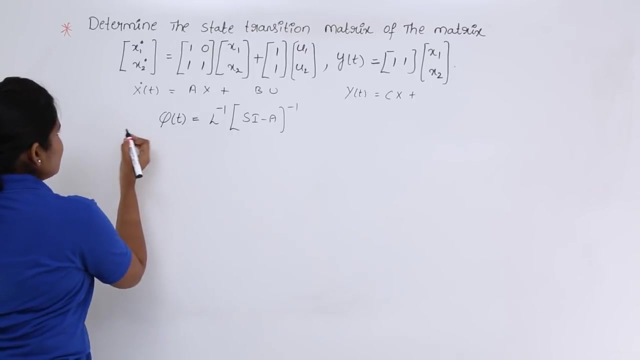 equation for state transition matrix. If you know S? i minus a whole inverse, then by taking inverse Laplace transform we can easily find out this state transition matrix. So first of all I want to know what is the value of S? i minus a? So here I know the value of a. 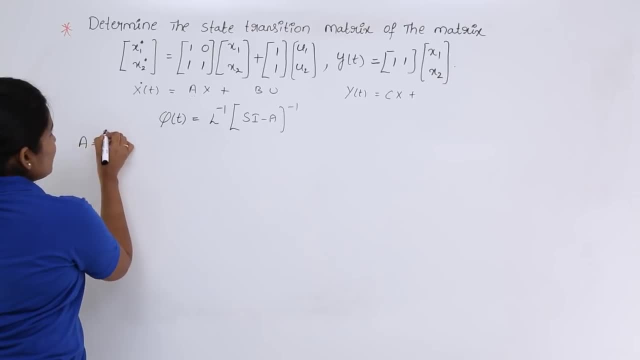 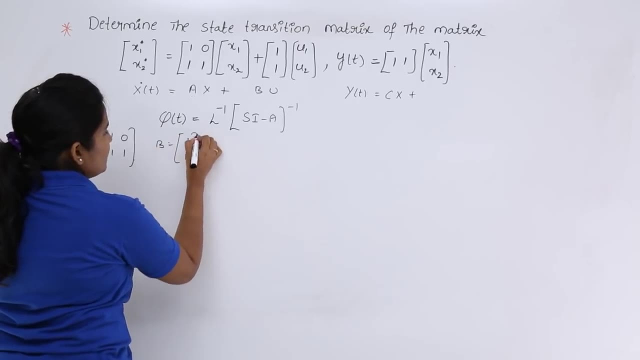 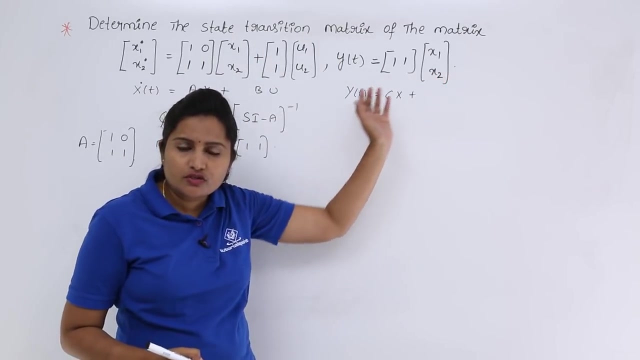 a is equivalent. I am writing the known values: a is equivalent to 1: 0, 1, 1 and b is equivalent to 1: 1 and c is equivalent to 1: 1.. Here, by the given model, can you see that is multi input, multi. 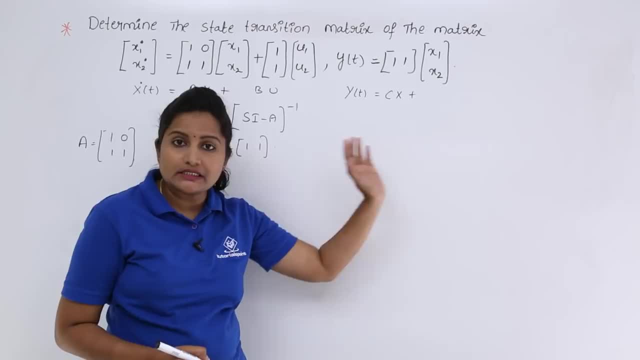 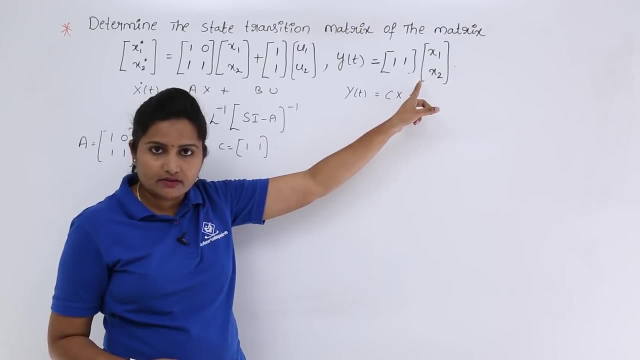 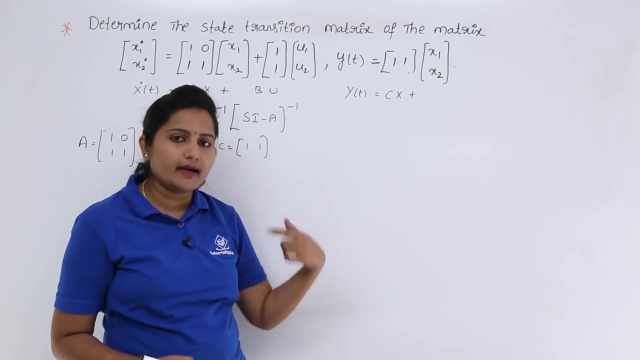 output system. This is multi input, single output system. If you see, this y of t is having only one line. this is not 2 by 2 matrix. So this is multi input, single output system. If you are having analysis for multi input, multi output, we can also apply for multi input, single output also. 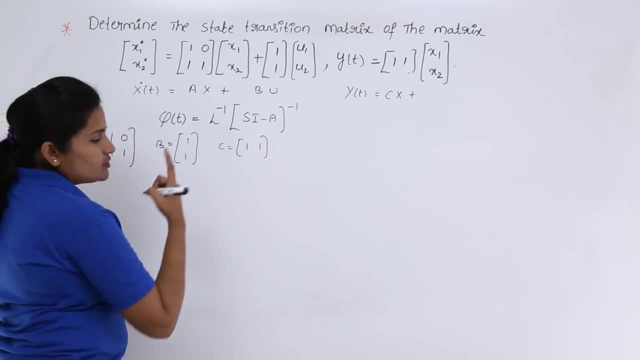 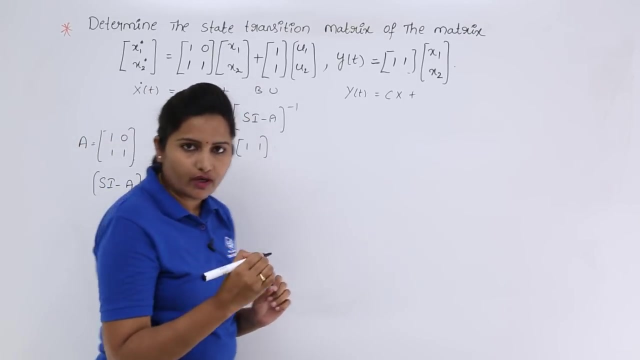 So here, a is equivalent to this, b is equivalent to this, c is equivalent to this, according to our given model. And now I am going to consider S i minus a value- S i is nothing but S- into identity matrix 1 0 0 1.. So here I can write S 0 0 S. 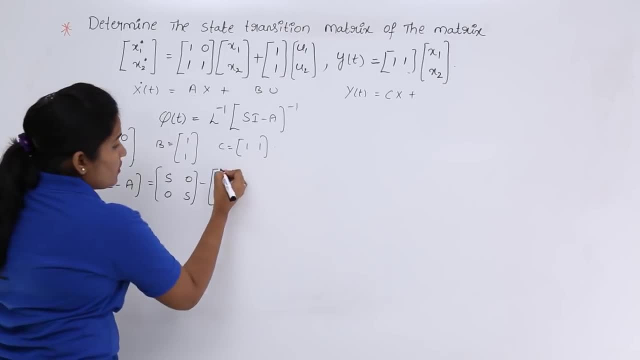 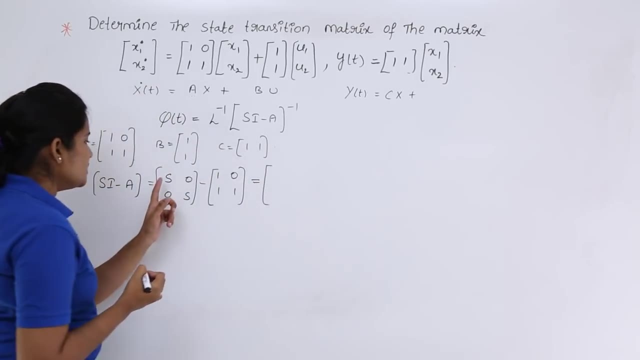 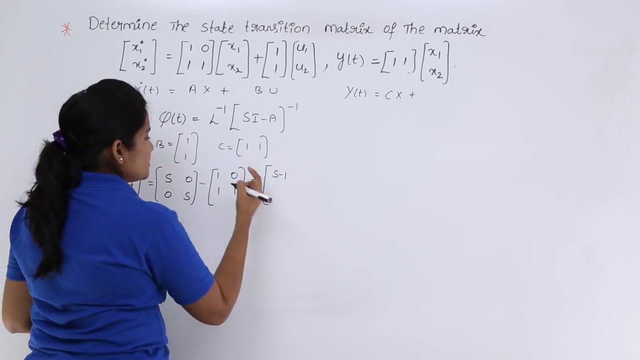 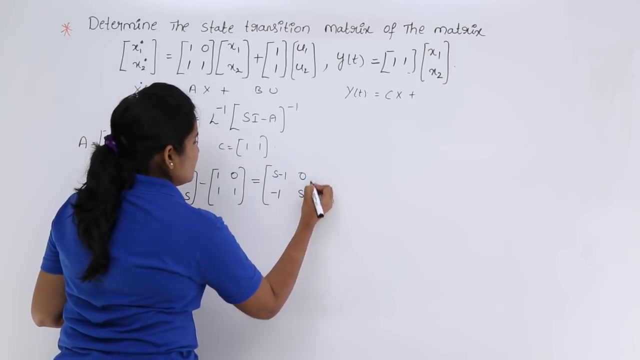 Minus a, a is this one: 1 0, 1, 1.. So S i minus a will give you like this. So this is nothing but S minus 1, and here 0 minus 0, 0 and 0 minus 1 minus 1, and S minus 1 will give you this: S i minus a. 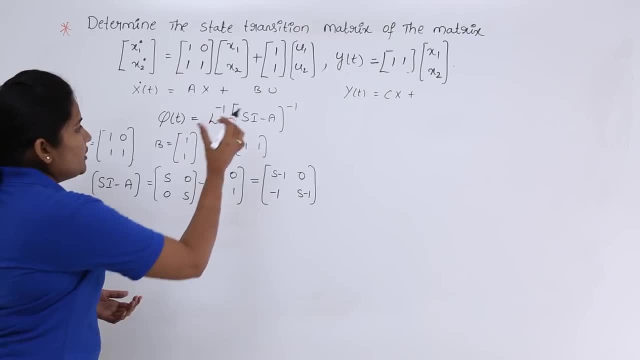 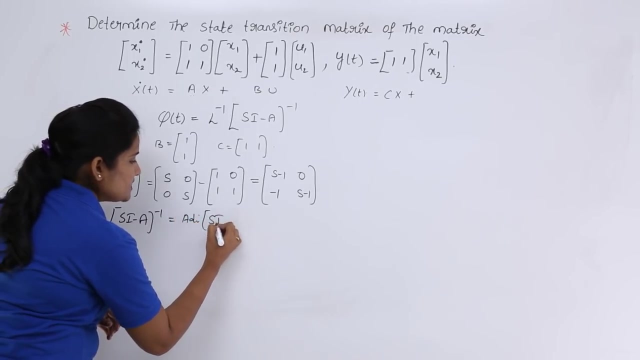 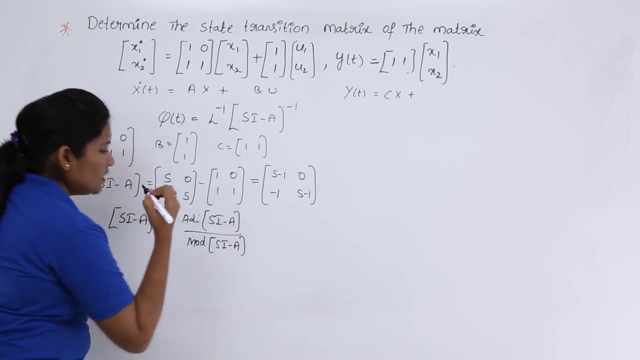 Now, from this S i minus a, if you want to get S? i minus a, whole inverse, we are having a formula That means to get inverse of this matrix, we need to perform a joint of S i minus a divided by modulus of S i minus a. Now I will derive these two, I will calculate these two and I will. 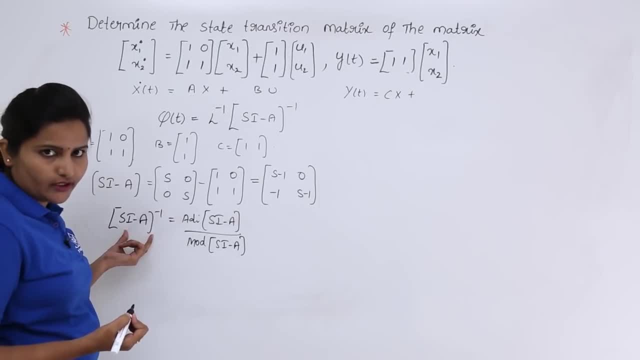 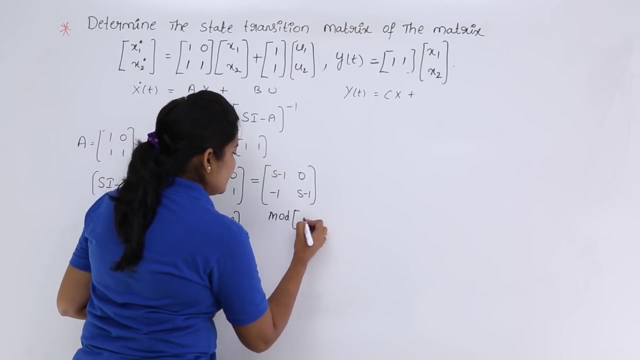 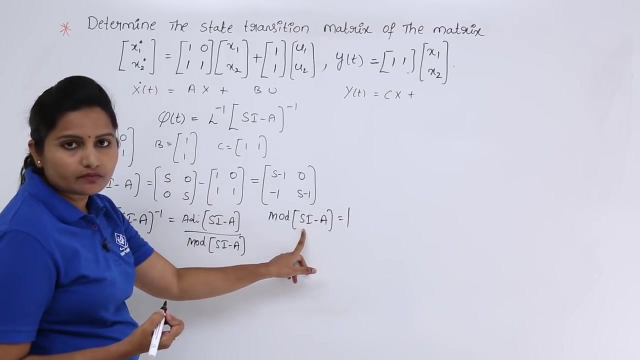 substitute in this formula, I will get S? i minus a, whole inverse, That means inverse of this matrix. and after that, by taking Laplace inverse, then I supposed to get my state transition matrix. So now modulus of S? i minus a. So here modulus of S? i minus a means modulus of this one, So matrix. 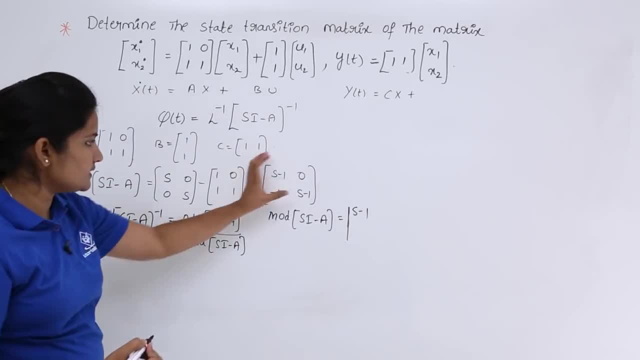 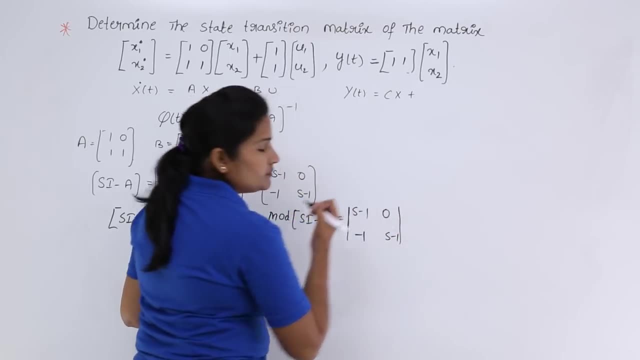 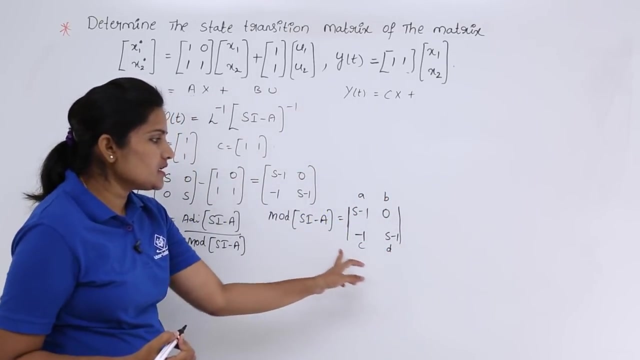 is S minus 1, S i minus a matrix. is this So S minus 1, 0 minus 1, S minus 1.. If you are having any matrix like a, b, c, d, so then modulus of this matrix will be: 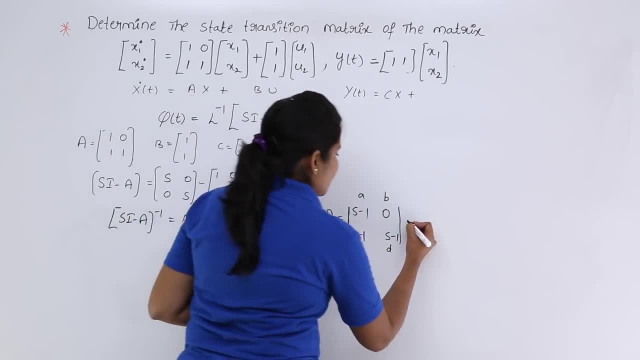 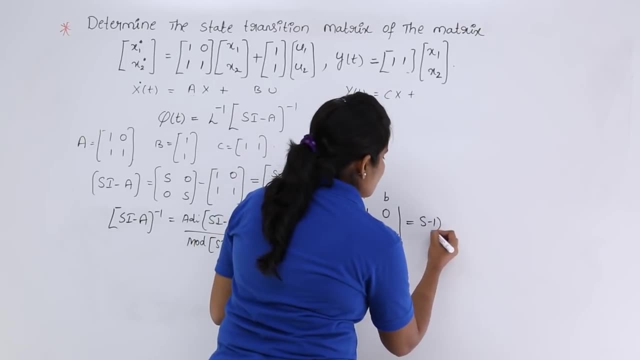 a d, e minus b c. So this is equivalent to the modulus of this S. i minus a is equivalent to a d. that means S minus 1. whole square minus means minus 1 into 0 is nothing but 0 minus of minus. 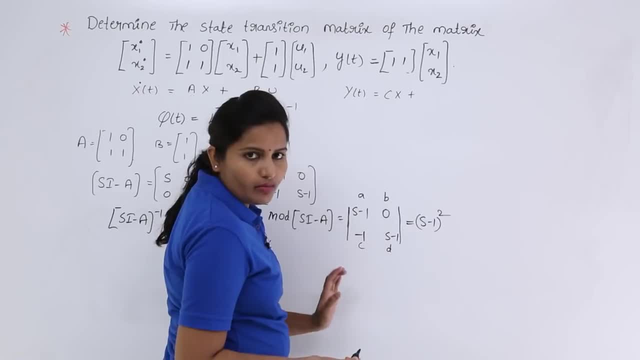 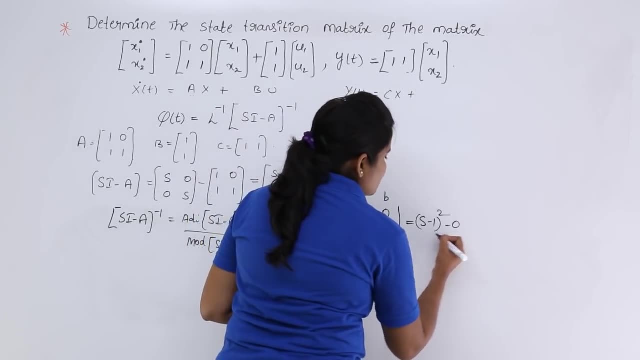 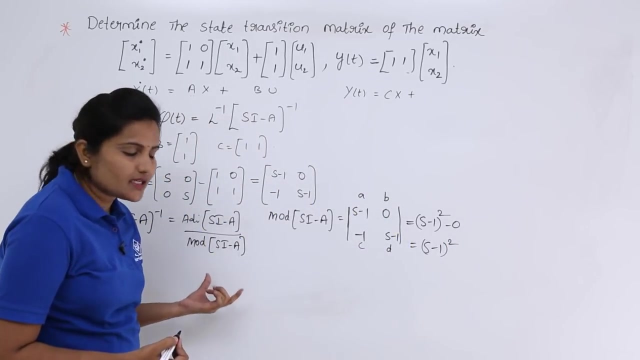 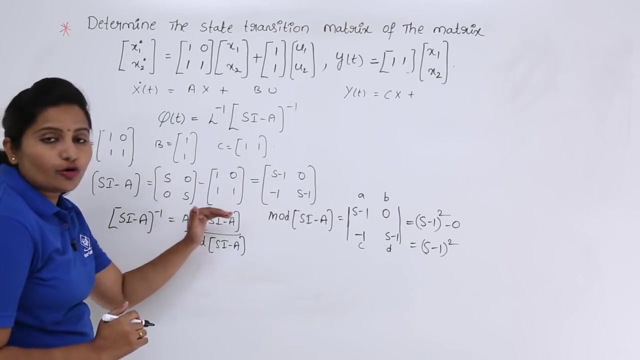 plus will. for example, if you are having any value, so minus of minus plus will take, but here 0 will be. there AD minus BC means so minus 0. so you will get only S minus 1 whole square. So here your modulus of SI minus A value will be S minus 1 whole square. Now we will calculate adjoint of. 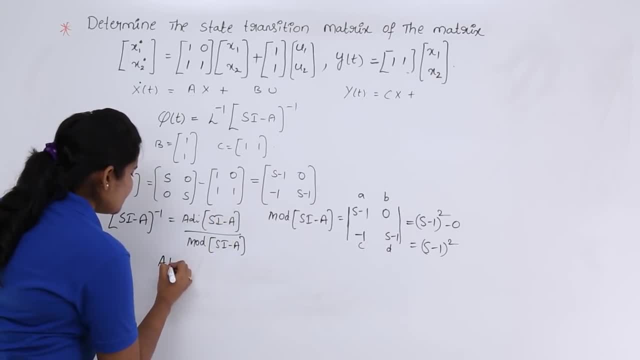 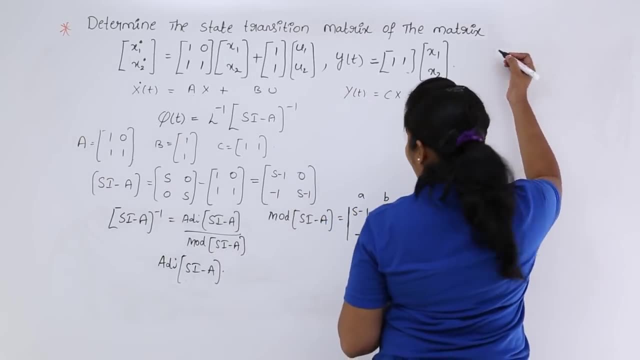 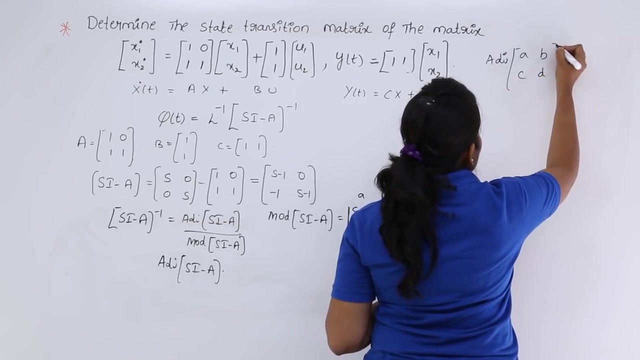 SI minus A. So for this adjoint of SI minus A. so to calculate this, for your reference I am giving you a formula. for example, if you are supposed to calculate adjoint of A, B, C, D, then the adjoint of A, B, C, D will be S minus 1 whole square. So for this adjoint of SI minus A, value will be S minus. 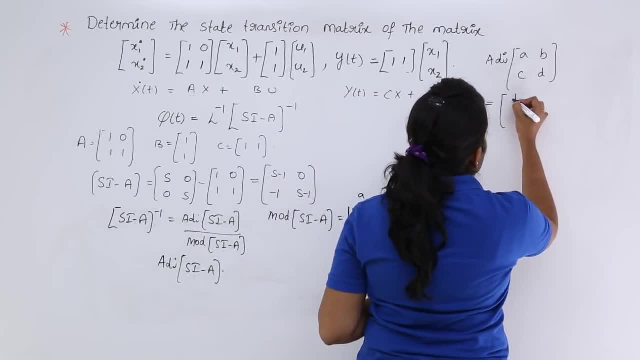 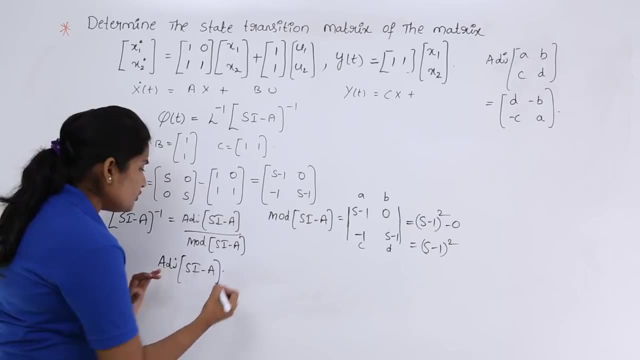 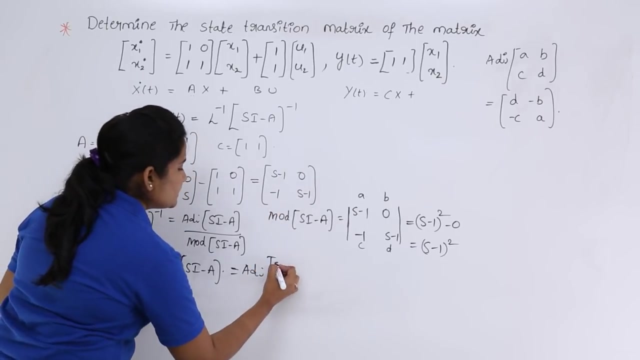 1. whole square D will be like this. So this is equivalent to D minus B, minus C and A. For example, if you want to write, adjoint of SI minus A means adjoint of this SI minus A matrix is S minus 1. 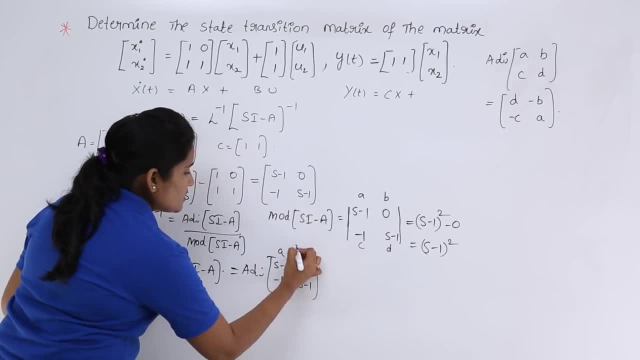 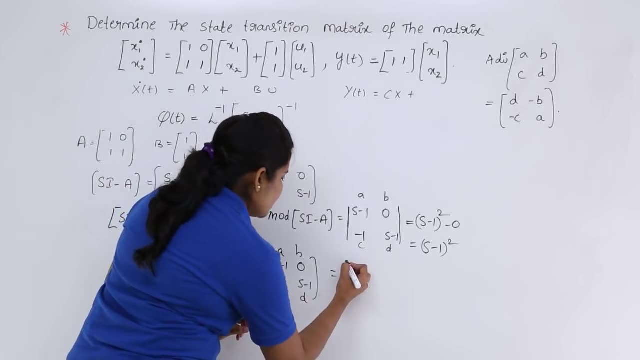 0 minus 1, S minus 1.. Suppose this is A, B, C, D, then when you are writing your adjoint, this will be like this: D, and when you will be writing into the A matrix, So you will get that. my detachment one call this: 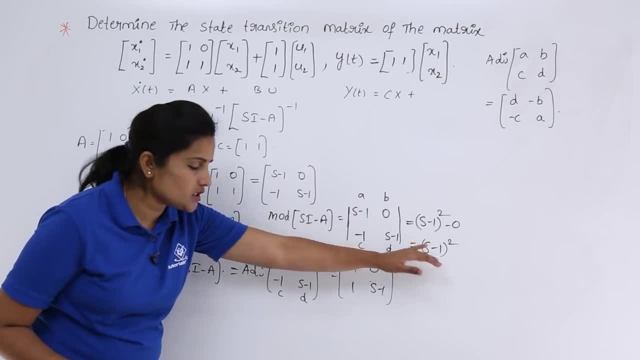 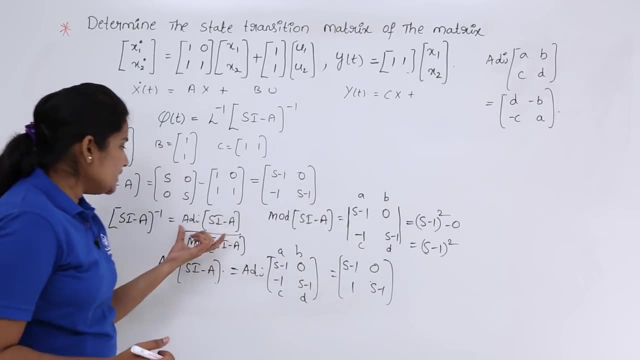 be ion, uh, which is A minus B. minus B is 0 only, So that will come as 0 only. and minus A minus A means less 1, and here you will get A. That means S minus 1, S minus 1, 0, 1, S minus 1.. Now we are. having both S minus 1 whole square and here adjoint of SI minus A. By taking these two in this equation we are going to get SI minus A whole square. So this is the norm of that and m1 total of A- S minus 1- is minus 3 punti, because at the moment this is general reef of A. This is our. 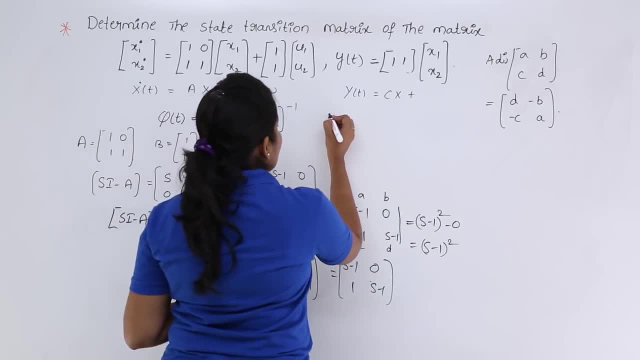 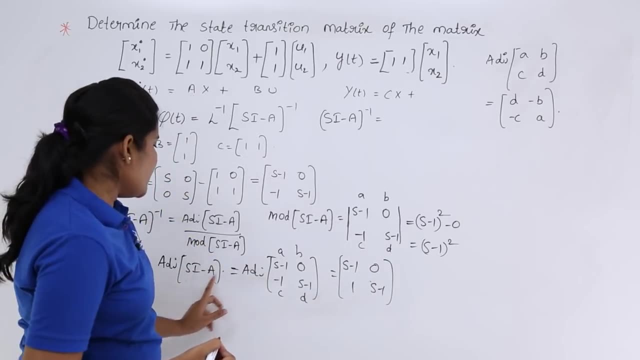 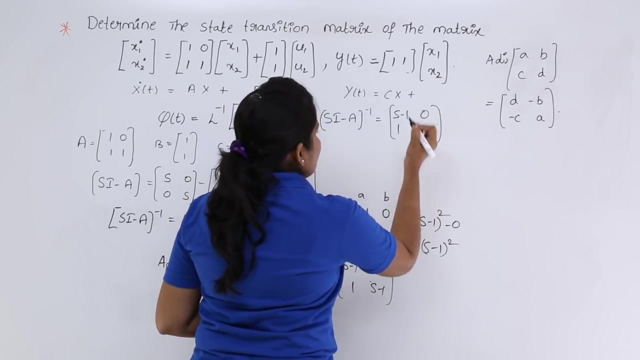 inverse. So now here I am going to write: S, i minus a whole inverse is equal n, 2.. So this one, so adjoint, is nothing but S minus 1, 0 and 1. S minus 1 and divided by you are having modulus. 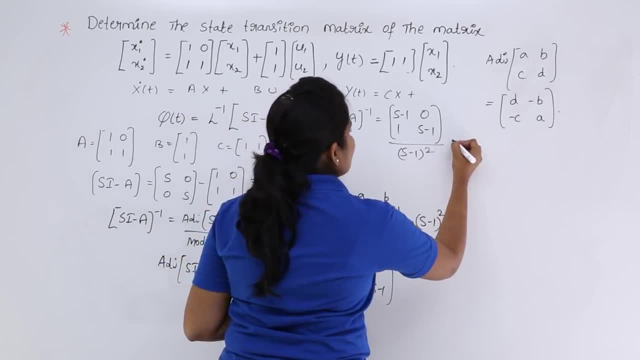 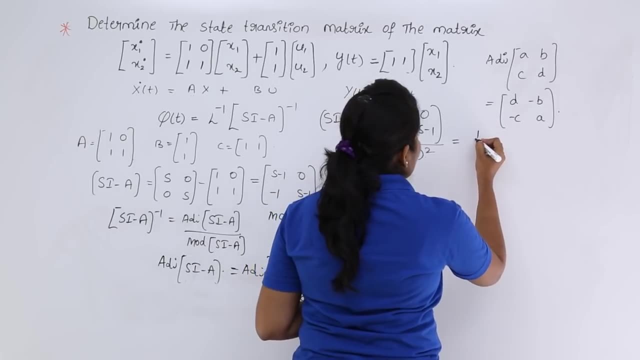 as S minus 1 whole square. Now this is equivalent to: so S minus 1 by S minus 1 whole square. So that is equivalent to 1 by S minus 1 and 0 by anything that is equivalent to 0. and 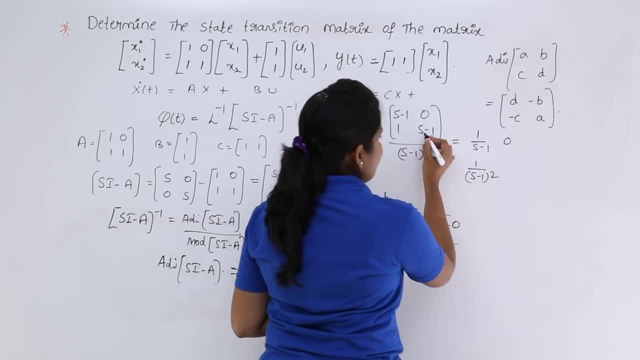 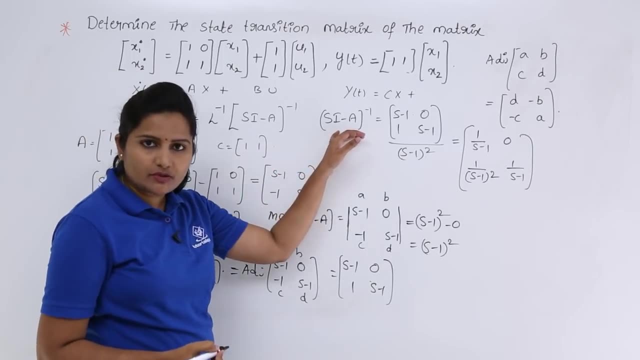 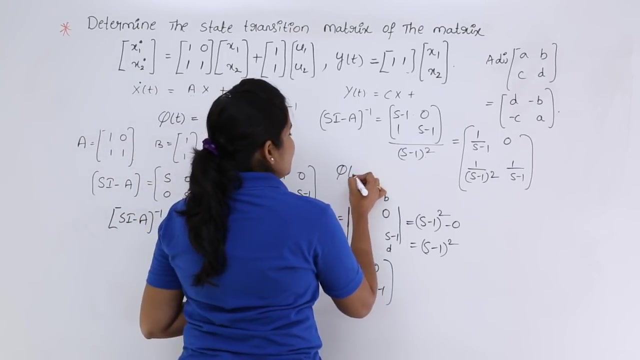 1 by S minus 1 whole square, and here also 1 by S minus 1.. This is the matrix we are going to get as your inverse matrix for your S i minus a. Now, finally, Finally, what we need to get. We need to get phi of t, that means state transition matrix. 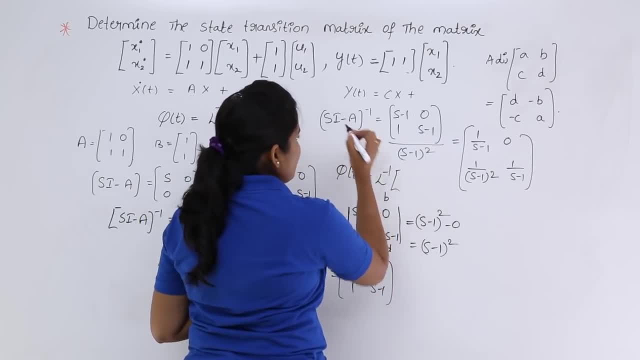 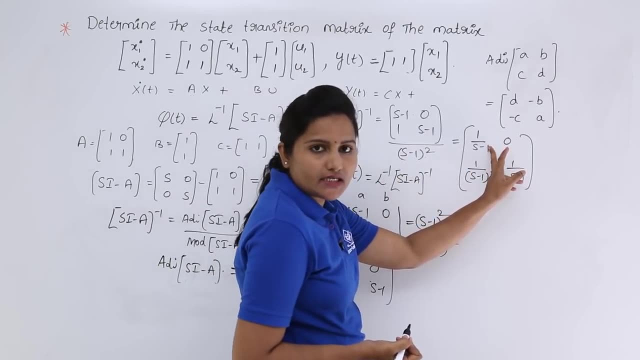 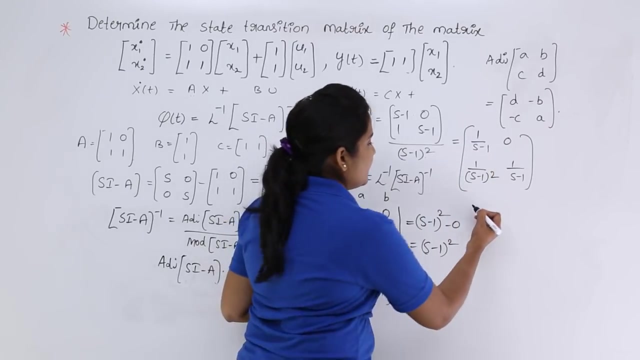 State transition matrix is nothing but inverse Laplace transform of this one S i minus a whole inverse. So now, if you take in inverse Laplace transform for this, if you see what is the inverse Laplace transform of 1 by S minus 1, that is nothing but e power t Inverse. 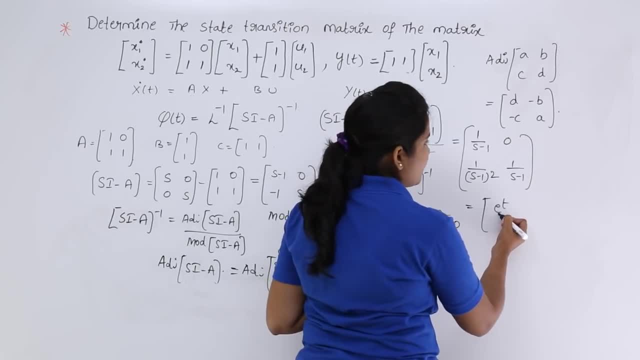 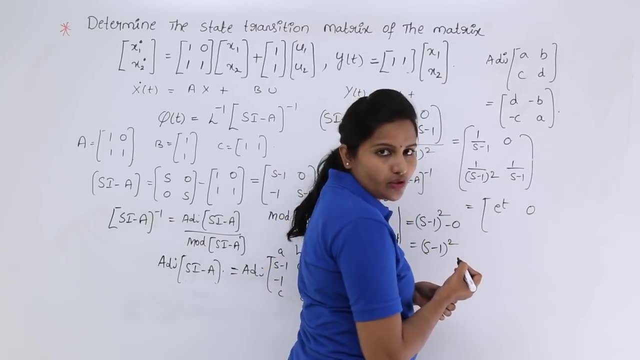 Laplace transform of S minus 1 by S minus 1 is e power t. And inverse Laplace transform of S minus 1 by S minus 1 is e power t. And inverse Laplace transform of 0 is 0.. And inverse Laplace transform of 1 by S minus 1 whole square t into e power.